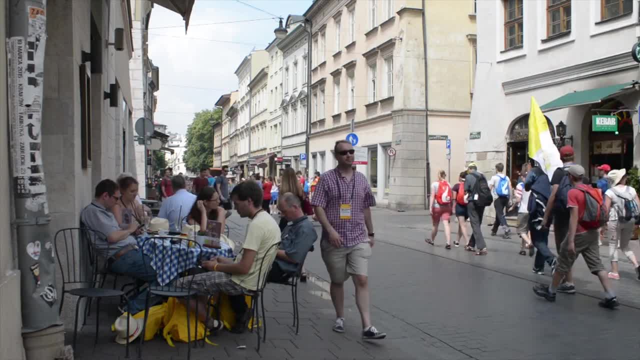 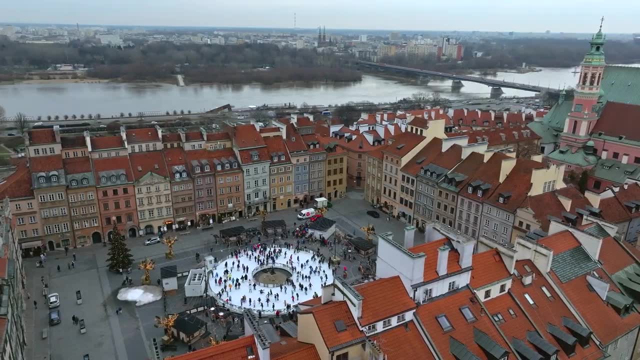 walk in the countryside. Winter is a great time to visit for those wanting to enjoy the festivals and events that occur throughout the summer, but unless you're here for those festivals, avoid the summer if you can. It gets very busy. Winter in Poland is very cold, but it can be a. 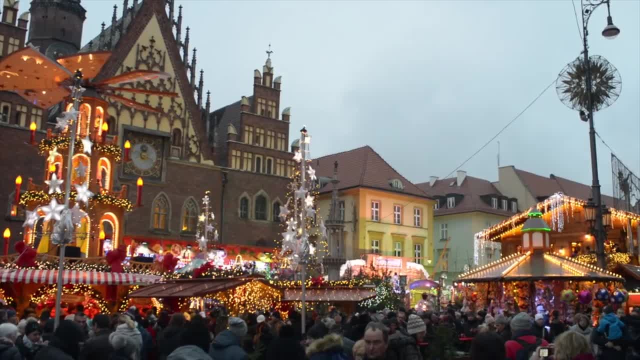 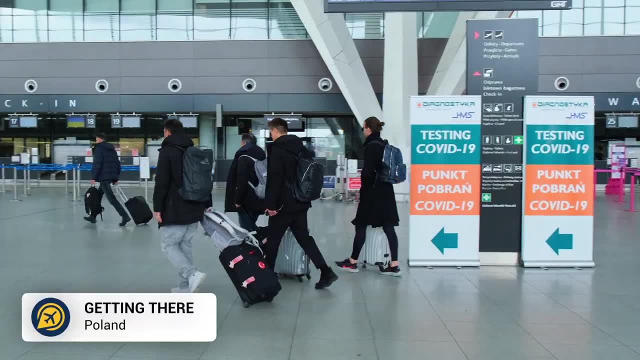 great time for the festivities and winter sports. Visit the major cities to enjoy the festive Christmas markets, but be prepared for the cold. So now let's look at getting there. Poland is well connected to other destinations in Europe, making it fairly accessible to travel to. 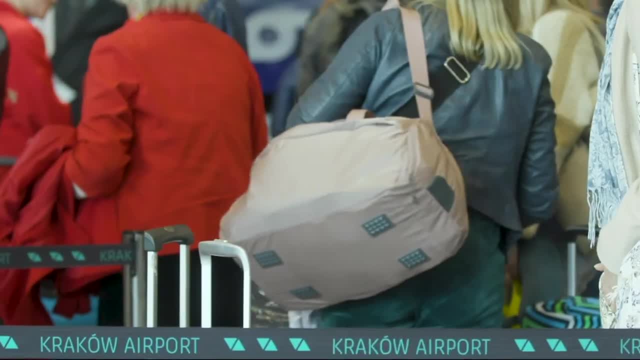 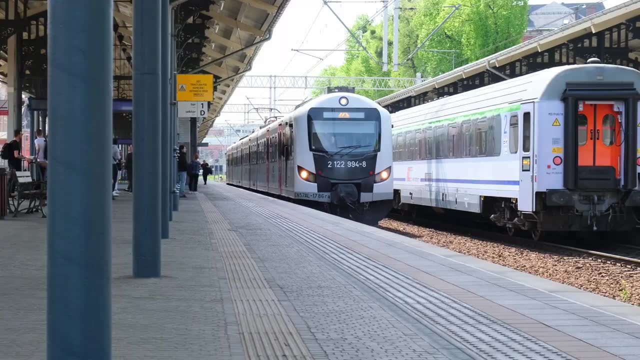 Depending on where you are in Poland, Poland is a great place to visit. Poland is one of the major cities where you can fly to one of the international airports in the major cities, with many direct flight options available to other destinations in Europe. Poland is also connected. 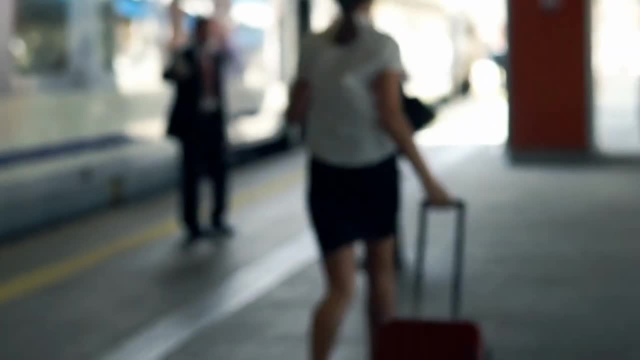 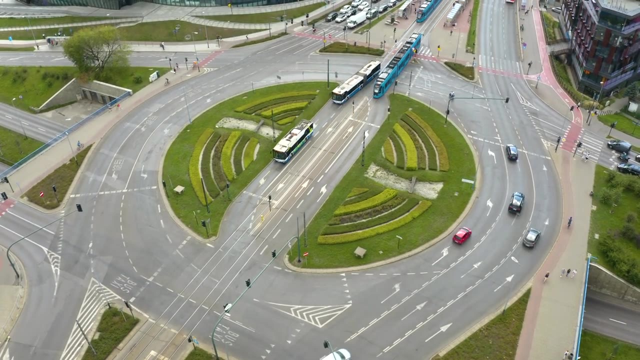 to neighbouring countries via train, so you can get here from Germany, the Czech Republic and Slovakia. You could also choose to take a long-distance bus from the nearby countries too. So now let's look at getting around. Travelling around Poland can be fairly easy. 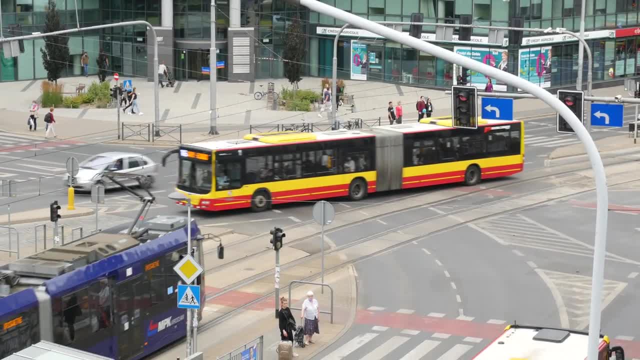 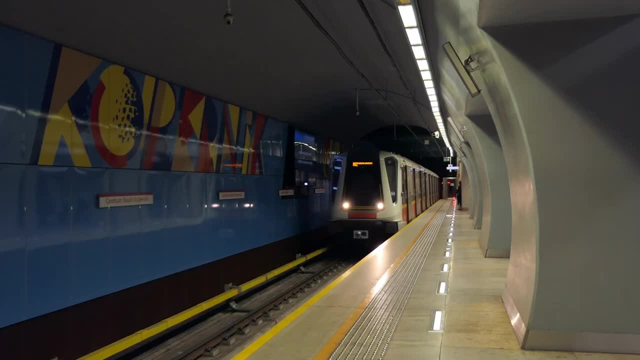 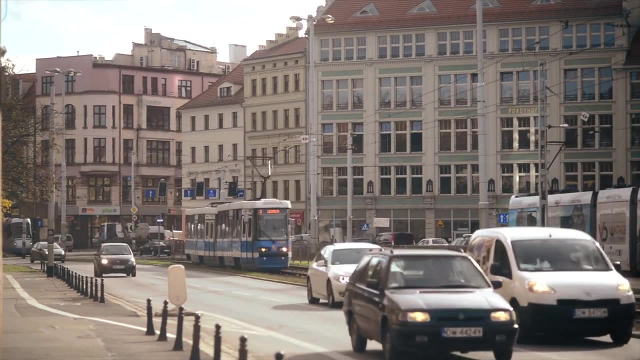 with a well-developed transportation infrastructure, giving travellers plenty of options. When you're in the cities themselves, you can use the trams and buses to get around. whilst Warsaw has a metro system to help you get around during rush hour quickly and efficiently, You can also use the taxi services in the city, especially helpful for 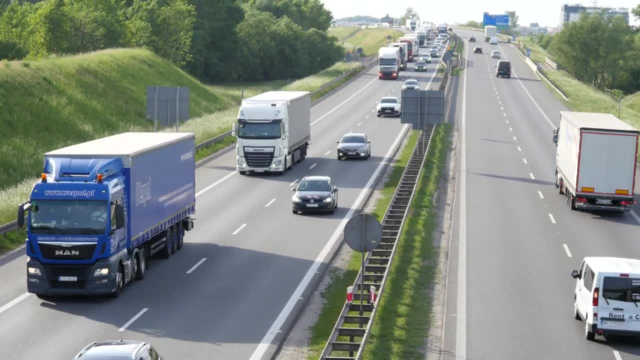 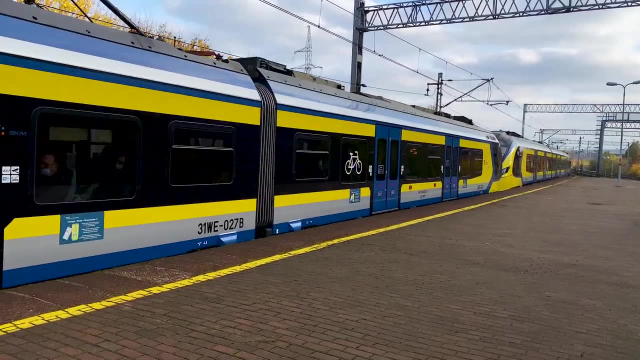 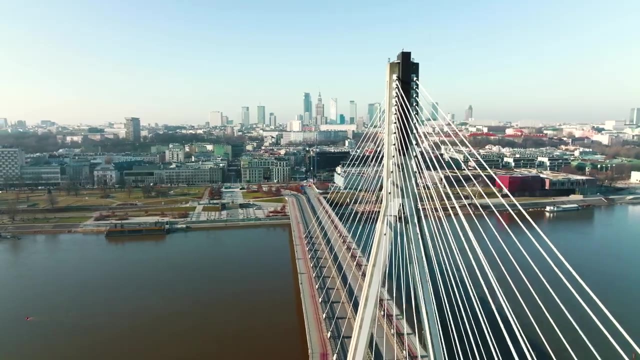 shorter distances. Travel between the cities and towns in Poland varies depending on the location, but rail travel is a popular, comfortable option, connecting most tourist destinations and offering express, high-speed options too. You can also use companies like Flixbus to get between the cities themselves. Of course, you could also rent a car if you want to visit the smaller towns and more rural areas of Poland. So now let's look at typical prices. Hostels in the major cities offer budget rooms from under 250 Zloty, whilst mid-range rooms cost around 360 to 500.. There are plenty of high-end. 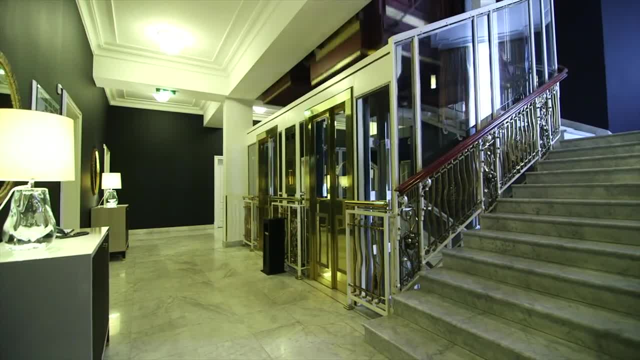 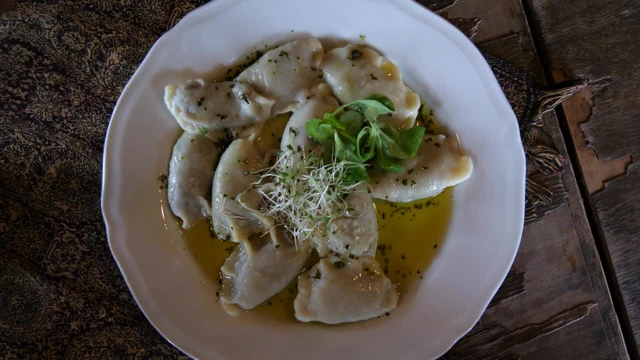 luxury options in the city, with a five-star hotel in Warsaw beginning at around 650 Zloty. A coffee and pastry from a Polish bakery will cost around 10 Zloty and a local meal or fast food can be found from under 45.. A sit-down meal including a beer or two will 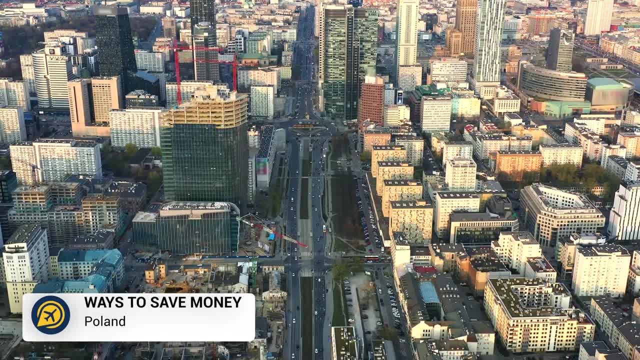 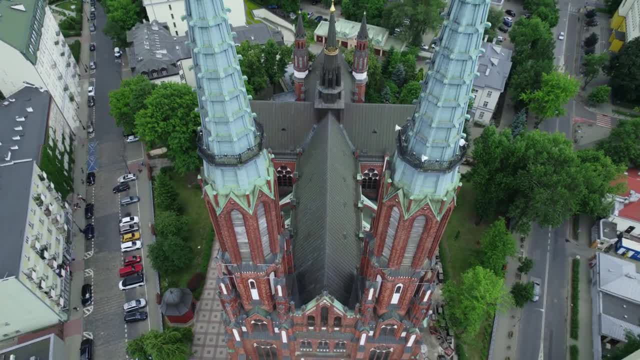 begin around 60. So Poland is a fairly inexpensive place to visit in Europe compared to its neighbouring countries. but there are many ways to save money as well: Visit in the shoulder seasons, from April to June and September to October, when the weather is warm enough to enjoy the free outdoor attractions, but you will also find cheaper hotel rates. You can take advantage of the budget airlines offering flights to Poland, such as Wizz Air and Ryanair. just make sure to book those flights in advance. Eat as much local food as possible. This is delicious, but also the more affordable options.